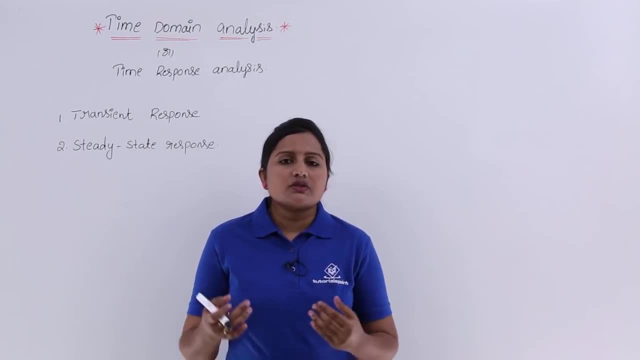 so response is nothing but output of the system. So time response analysis is nothing but variation of the output of the system with respect to time is called as time response analysis. That means so if time is varying So with the time, what is the variation? 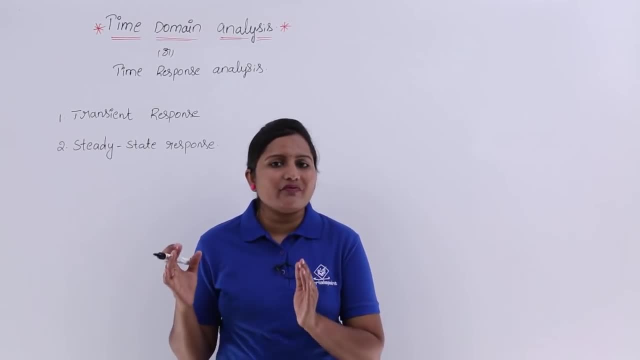 of output of a system. So that means we need to see the variation of output C of t. So that is called as time response analysis. With this time response analysis we can study the variability of the system, accuracy of the system. So we can study the system by using this time. 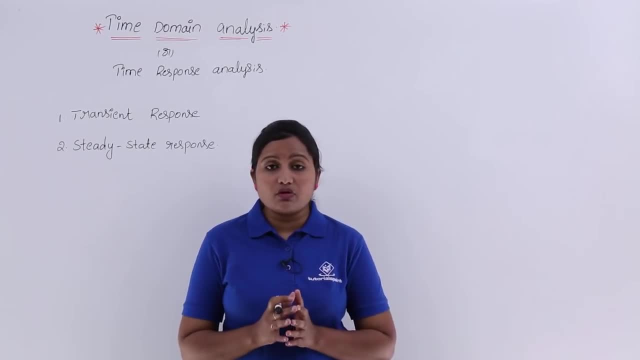 response analysis. So this is very important throughout control system: How we will calculate this. time. response means time. response is nothing but output with respect to time. So up to now we discussed our output in terms of transform. That means we consider as frequency domain frequency domain of the output. 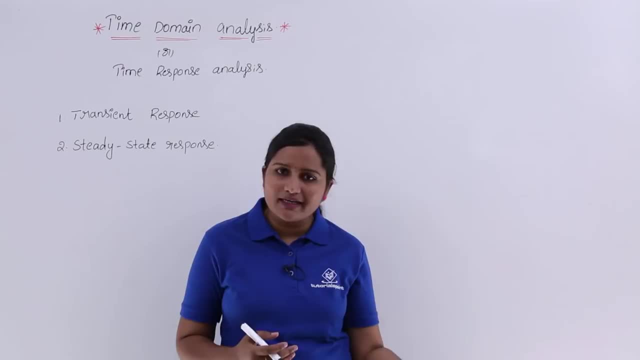 to now. we consider in our previous videos to calculate transfer function or gain. so that means you consider c of s, but here time response analysis. so you are going to calculate your output with respect to time, so that that is meant by the output in time in terms of. 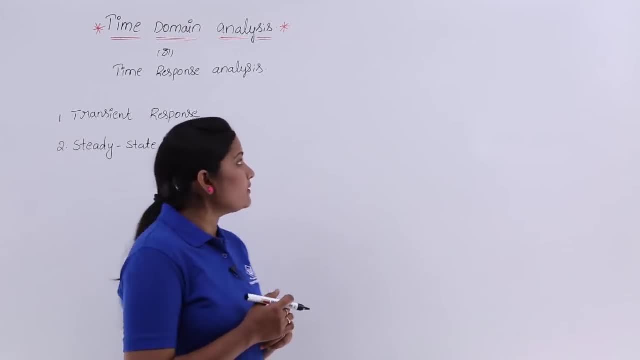 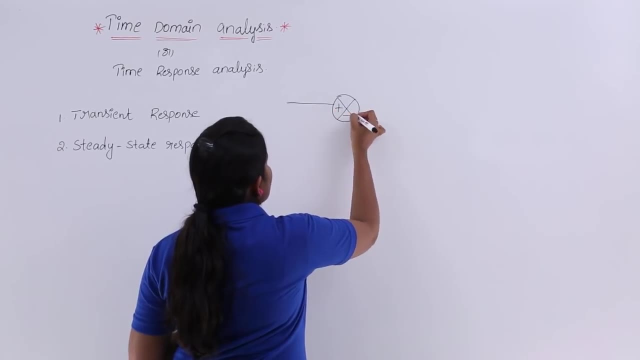 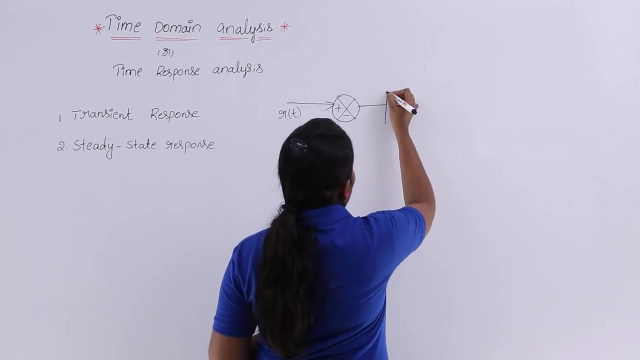 time c of t you are going to calculate. so here i am going to consider a control system. so here i am having a control system like this. so here i am giving a signal r of t. so now, here i am having a gain- ah, this is open loop gain g of s. and here you are having c. 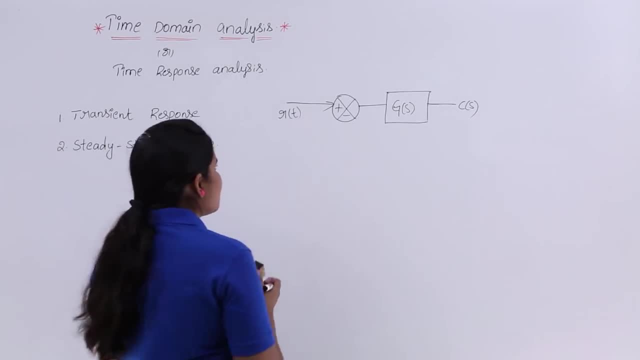 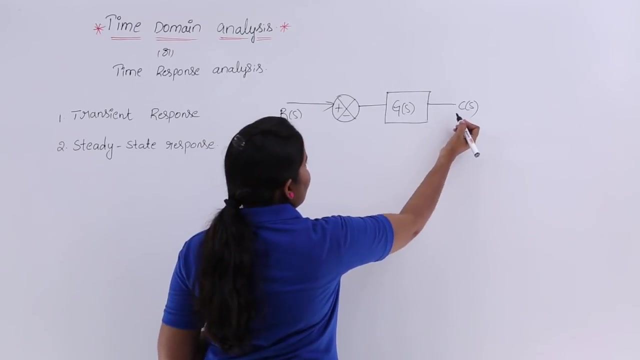 of s. so here, as previous, you just consider: like a transforms why? because you are ah open loop gain and forward path gain if they given in terms of laplace transforms. so here you are having a transform. then here r of s is the input transform, output transform, open. 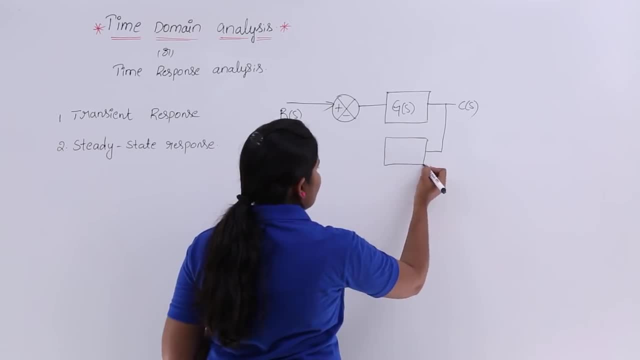 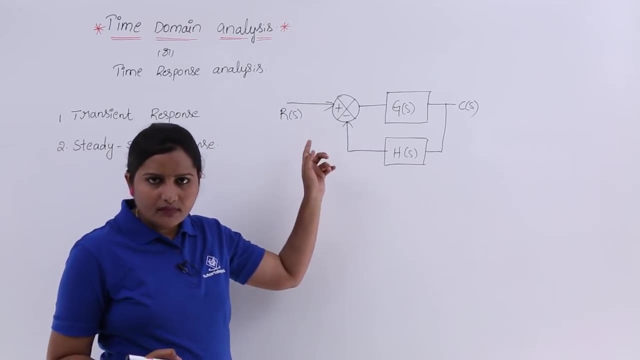 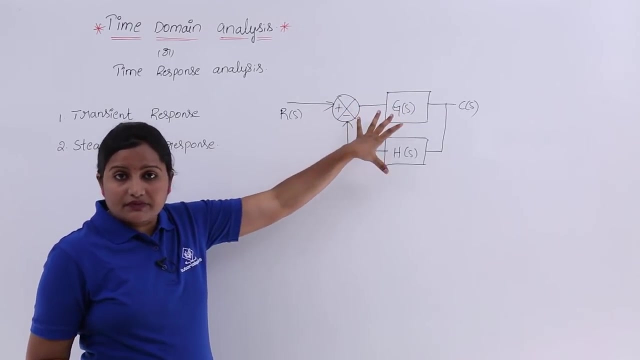 loop gain and feedback gain. if you consider that is equivalent to h of s. so you know this is a negative feedback control system. you know this is a negative feedback control system. for example, if you want to do time response analysis for the system, you need to find out. 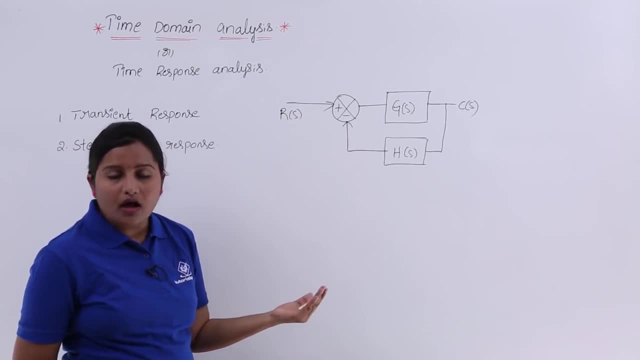 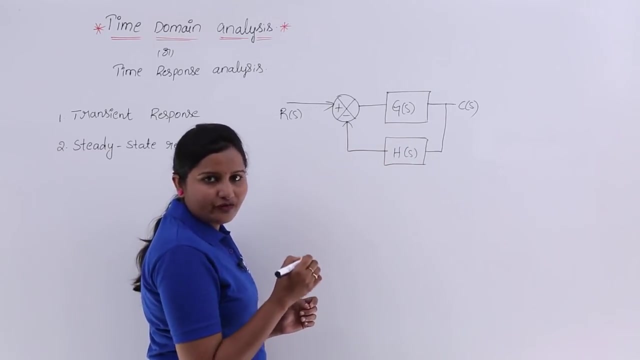 the output. so how will find out the output? how you will find out the time. response analysis means so you need to get the output. with respect to time, that means you need to get c of t. so here you know that from the knowledge of negative feedback system, you know that the transfer function t of s is equal into c of 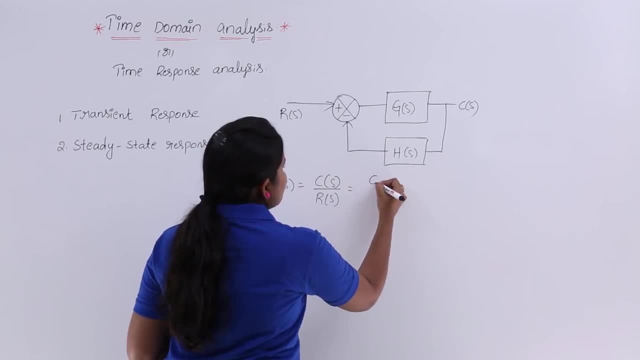 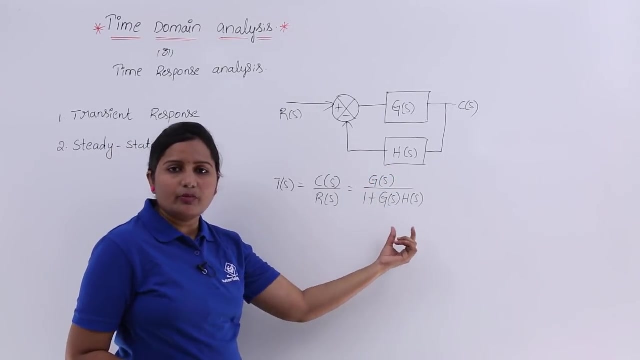 s by r of s is equal into: so g of s divided by 1 plus g of s, into h of s. so this is the transfer function of this negative feedback system. so that means: so open loop gain divided by 1 plus open loop gain into feedback gain. so this the transfer function of negative. 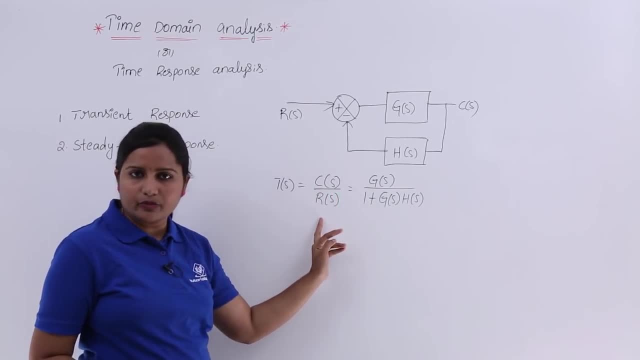 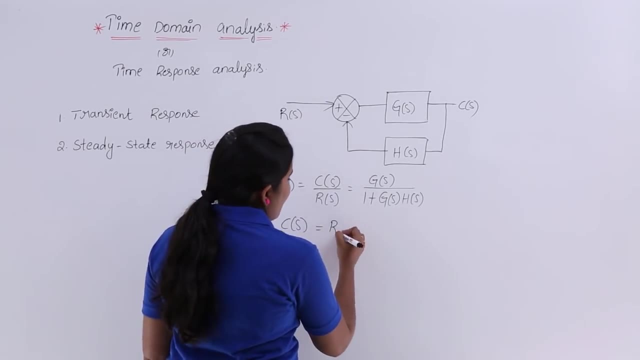 feedback system transfer function is nothing but output transform by input transform. so by this i can write the equation for c of s. c of s is equal into r of s, into g of s, divided by 1, plus g of s into h of s, So ultimately to get time response. so how you will get so, time response means output. 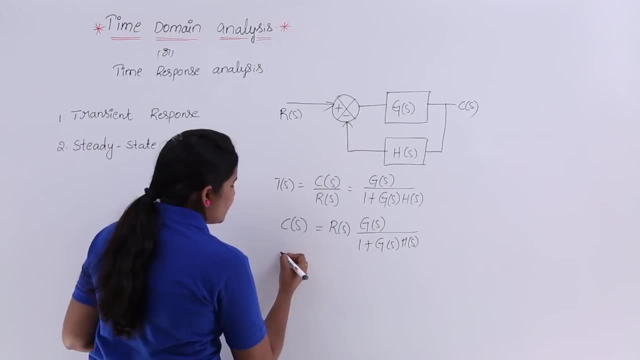 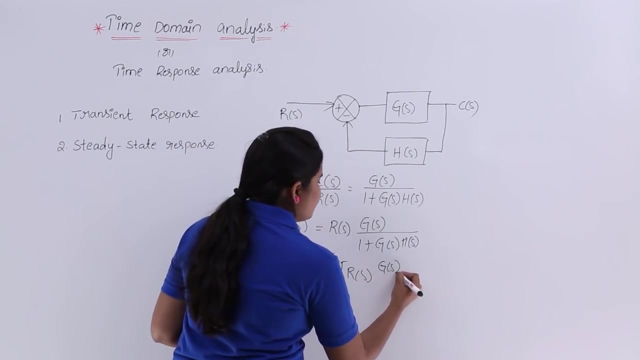 with respect to time, that means you need to get c of t. for that, take inverse Laplace transform on both sides so you will get. c of t is equivalent to Laplace transform of r of s into g of s, divided by 1, plus g of s into h of s. 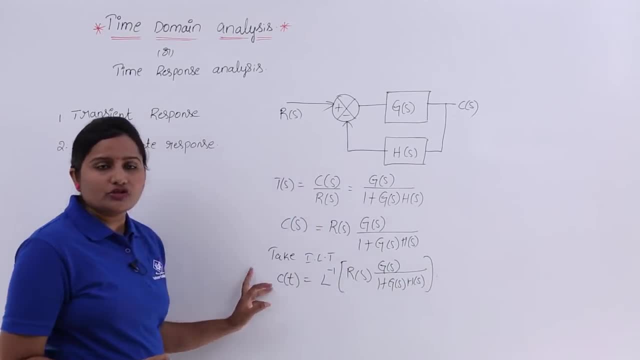 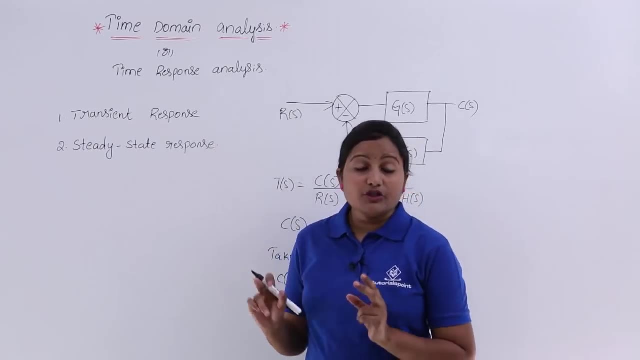 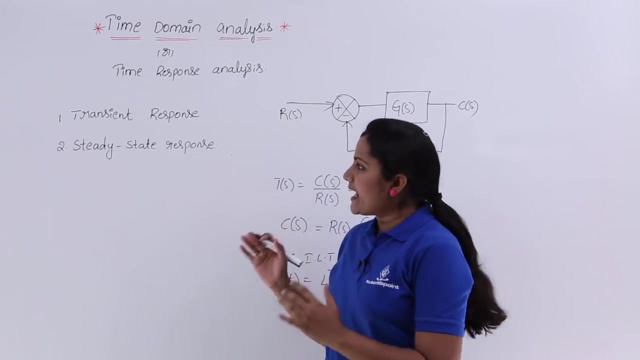 Like. this way we can get Our time response of the system. so now coming to types of response. so here we are having two types of time responses. that is, transient response, and second one is steady state response. so transient response is nothing but response of the system, which varies with time so coming. 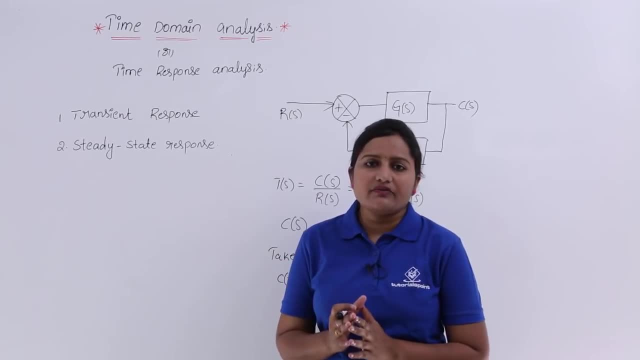 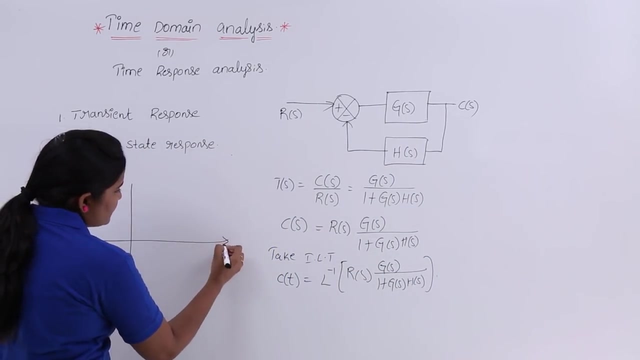 to steady state response. so steady state response of a system won't change with time, so it will come Constantly. so for example, if you are having, if you are having- any response c of t like this: this is t and on y axis I am going to consider c of t. if your response is like this: 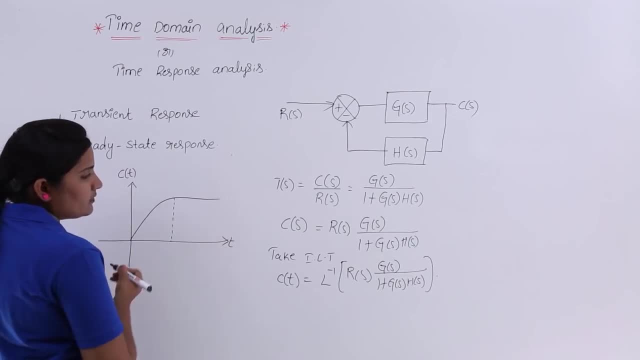 so up to here, it is varying. from here to here this is constant, so this is called as transient response. So From here to here, this is transient response of the system and steady state response of the system. from here to this constant value where you will get up to where you are going. 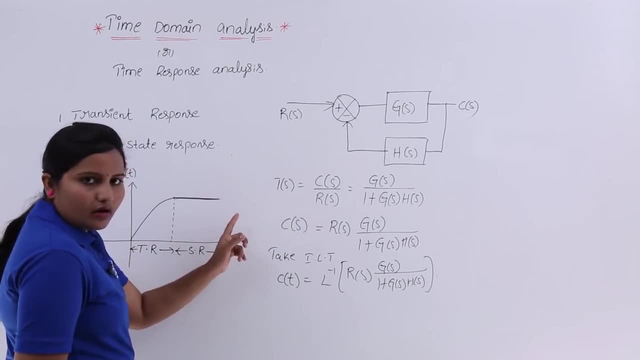 to get this constant value so up to that point. so that is steady state response. that means so you can observe here. so this response is varying with time. if you are increasing your time, this going to vary, But Here In this place, if you are varying time, also your response is not going to vary. it is like 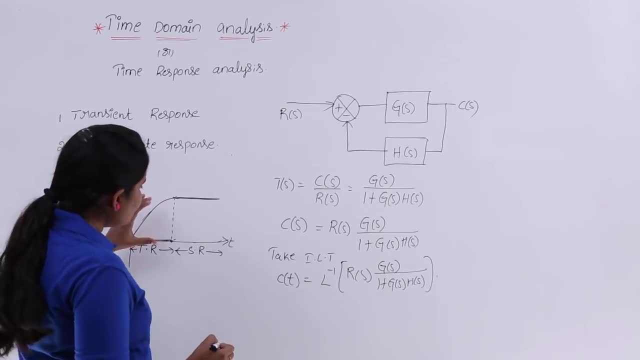 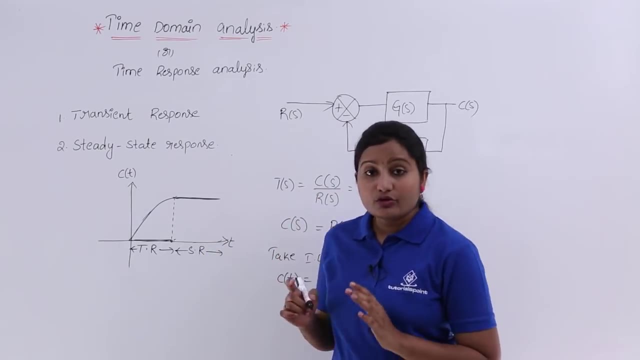 a constant. it's in steady state, so this is transient response. this is steady state response. we are having two types of responses here. so we will have two types of responses here. one is transient response, which varies with time, and another one is steady state response, which won't vary with time. as the name indicates, it will have a steady value, like this. so it's. 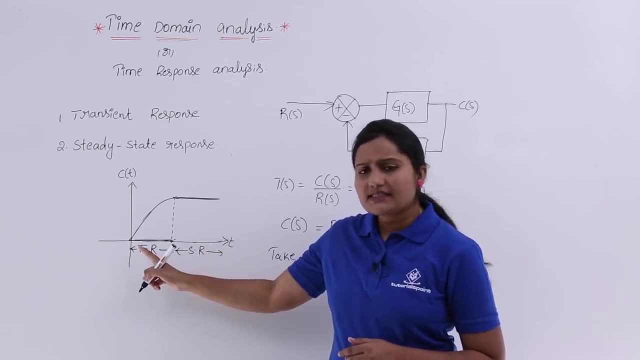 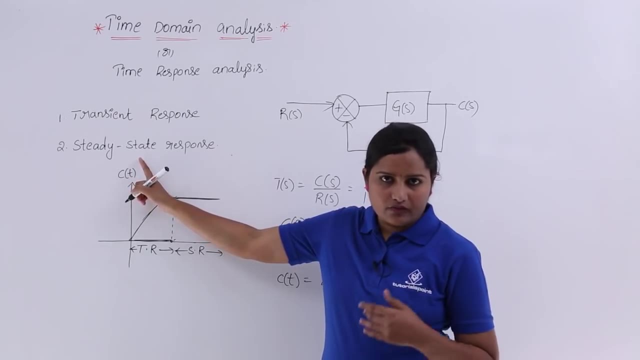 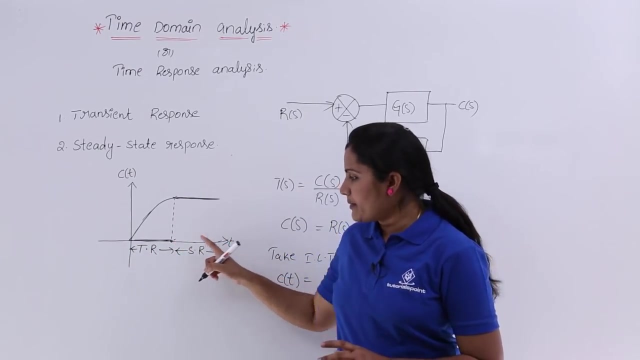 going to vary with time. So The best example response for these two responses is like this: if you are time, response or output of the system is like this: then up to here we can say that is a transient response, and up to from here to that steady state value, you will call that as a steady state response. 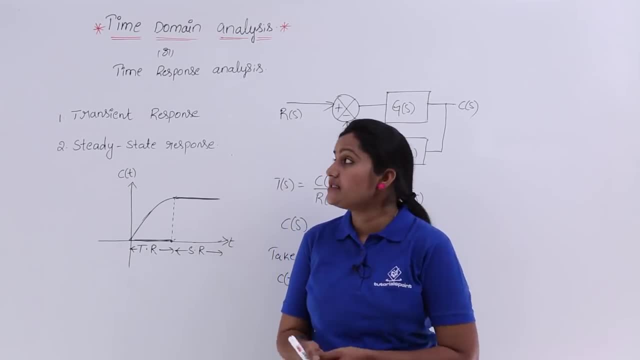 this is about introduction of time domain analysis and time or time response analysis. we can call it as time domain analysis. So This is very important, very important chapter, you can say in terms of gate. so we will get some two marks questions, one mark questions from this unit. so this introduction is also 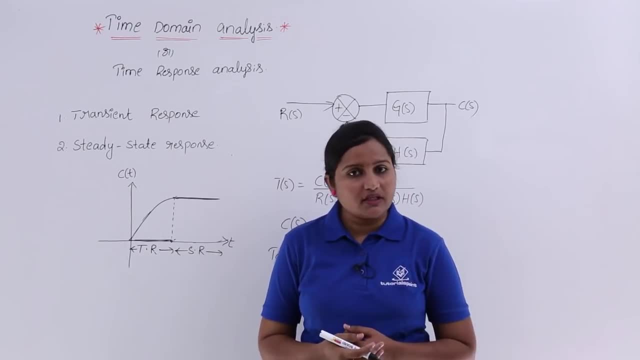 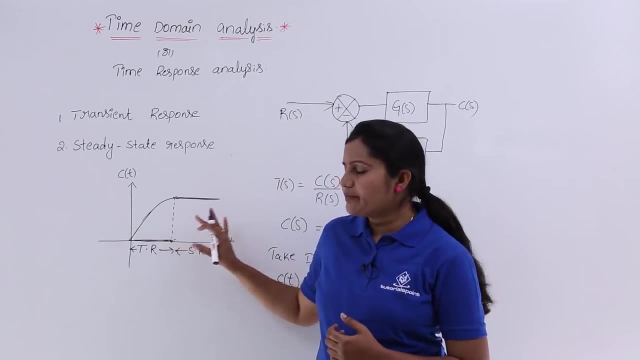 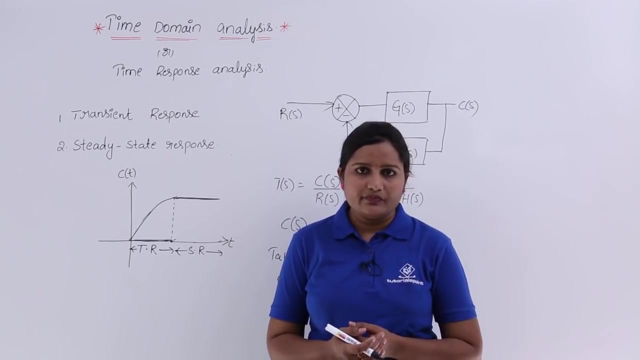 very important. so how many types of responses we are having, that point is also very important. so you just need to know the difference between transient and steady state. So this is the simple difference between transient and steady state. This is about the interval, This is about the interaction of time. domain analysis.